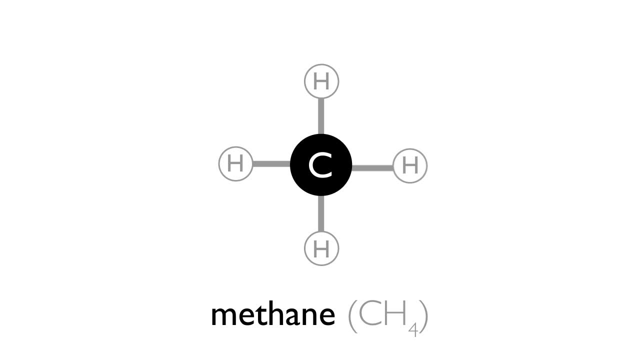 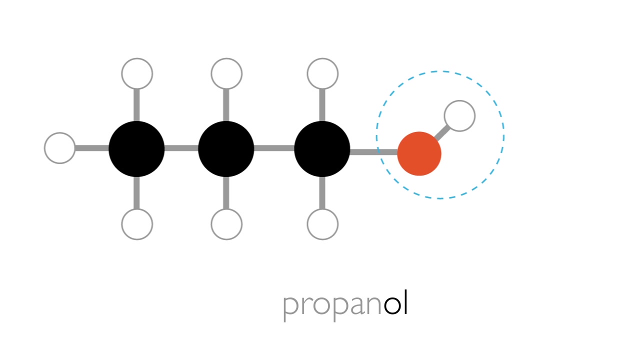 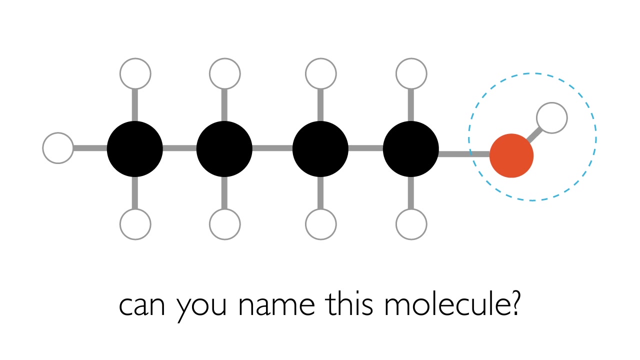 Here is methane. Replace a hydrogen with the alcohol functional group to form methanol. Here is ethane. And here is ethanol, Propane and propanol. Pause the video and name this molecule. This was butanol. Did you get it right? 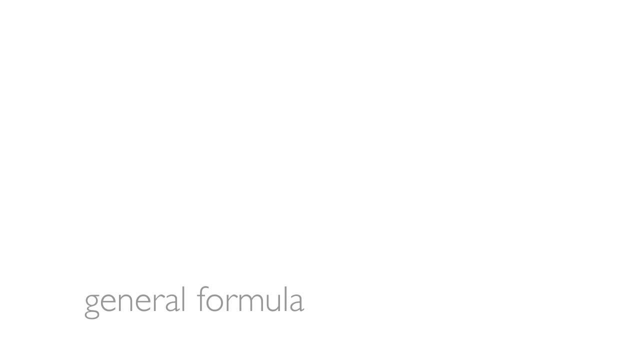 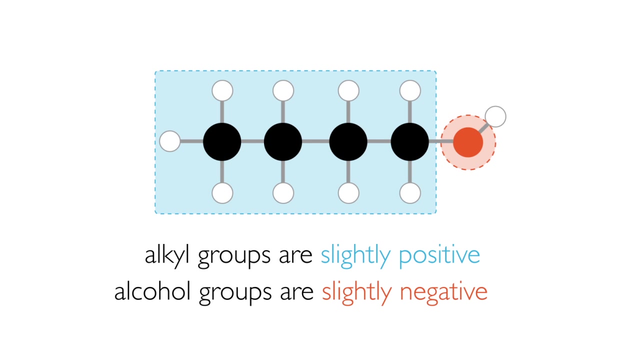 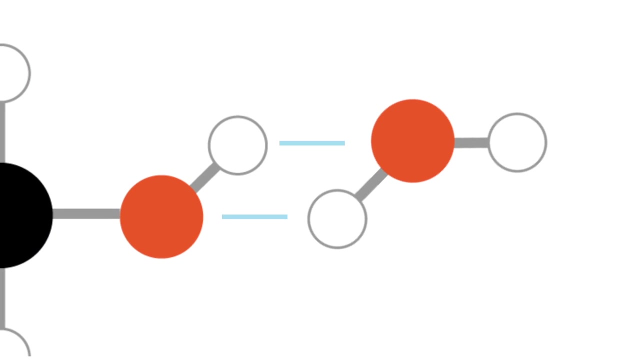 The general formula of the alcohols is CnH2n plus one OH. The OH group is an alcohol group with the hydroxyl functional group. The OH group generally makes alcohols polar molecules. The hydroxyl group also gives rise to hydrogen bonding. 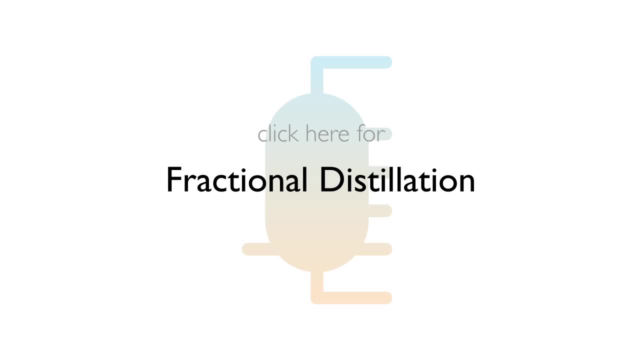 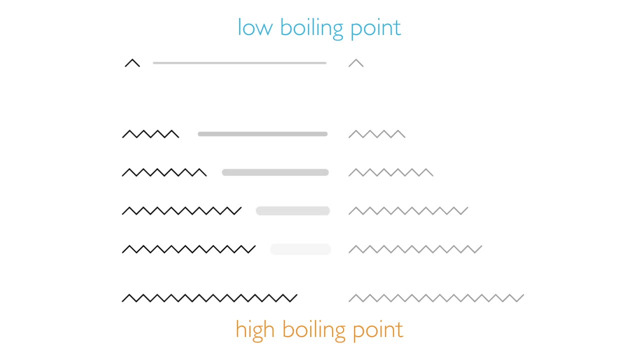 In our video on fractional distillation, we discussed how increasing chain length increased the boiling point due to increased intermolecular forces. The alcohols follow this same trend, but their boiling point is even higher than their comparable alchemes, and this is due to the hydrogen bonding. 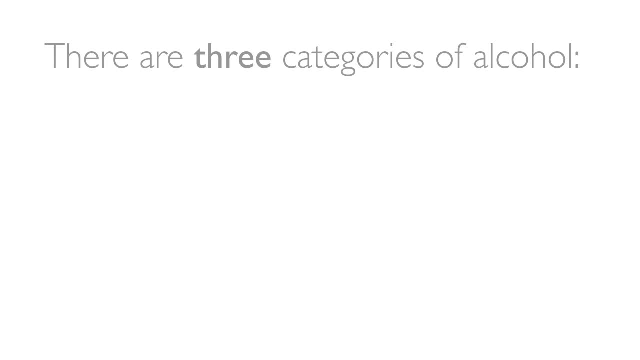 Alcohols are placed in one of three categories- Primary, secondary or tertiary- based on the position of the OH on the chain. Alcohols will react differently depending on the category they are in. In a primary alcohol, the carbon atom on which the OH group is bonded is itself attached to only one carbon chain or one alcohol group. 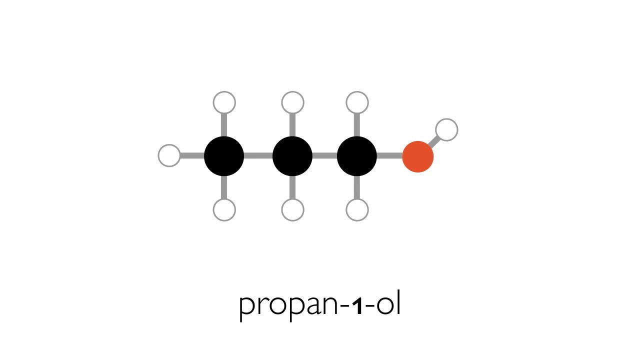 Here is propanol. The OH is attached to the end carbon and this carbon is attached to just one single chain of carbons. In secondary alcohols, the carbon atom on which the OH group is bonded is attached to two carbon chains or two alkyl groups. 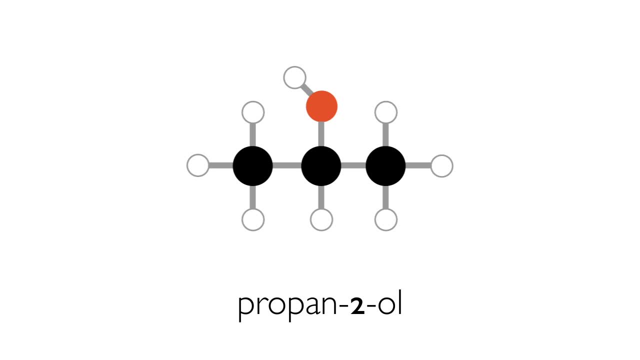 Here is propan-2-ol, Here is the carbon atom on which the OH is attached And here you can see the two alkyl groups or two chain groups. In tertiary alcohols there are three carbon chains attached to the carbon on which the OH group is attached.